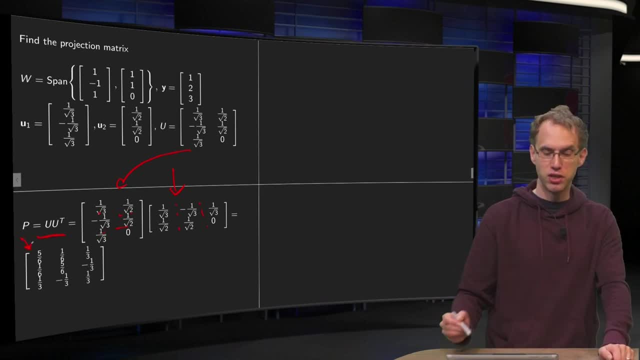 So 1 over 3 plus 1 half equals 5 over 6.. That is the first element, And the second element is minus 1 over square root of 3 times 1 over square root of 3.. Minus 1 over 3 plus that product over here, minus 1 over 3 plus 1 half gives us 1 over. 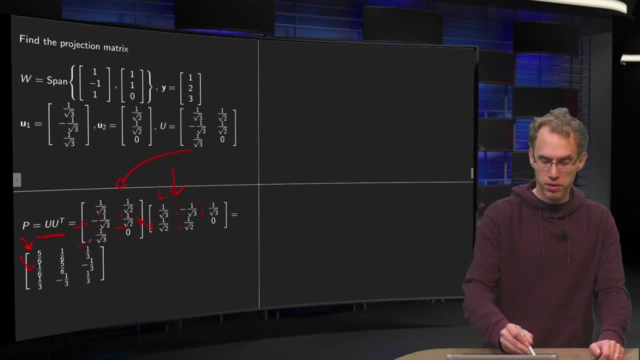 6.. Next term: 1 over square root of 3 times 1 over square root of 3 equals 1 over 3 plus 0 equals 1 over 3.. And there you have the first column and you can do the second and third column yourself. 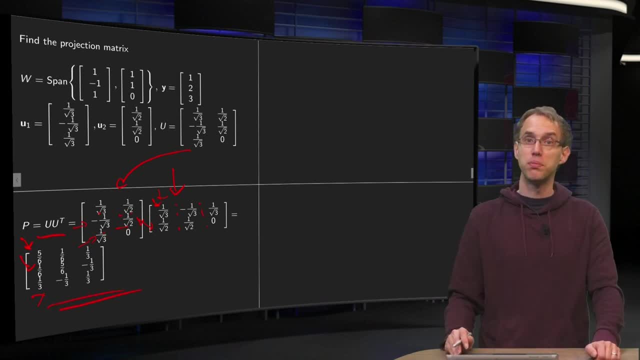 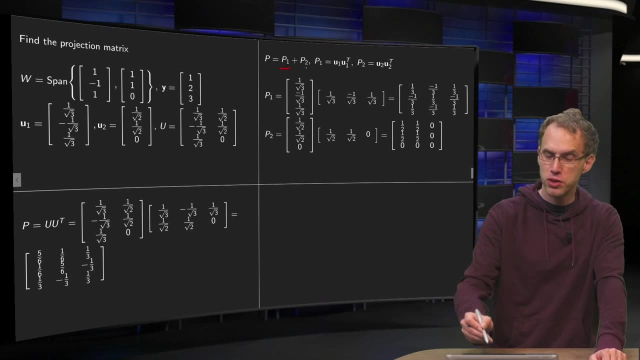 So there you already have a projection matrix p. Now let us do it in the second way as well. We can write p as p1 plus p2, where p1 equals u1 times u1 transpose and p2 equals u2 times u2 transpose. 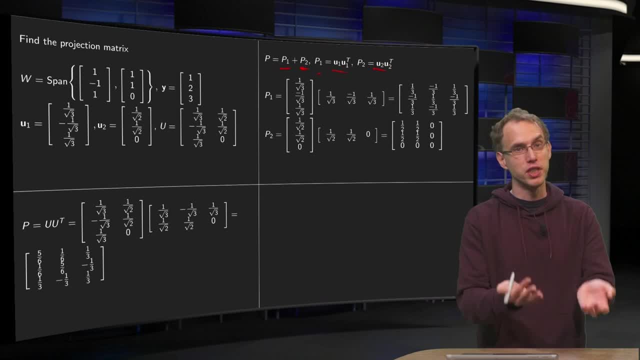 The advantage is that then your p1 will be the projection matrix onto u1, p2 will be the projection matrix onto u2 and the sum of the two will be the projection matrix onto w. So let us compute p1.. So here you have your u1 and your u1 transpose. 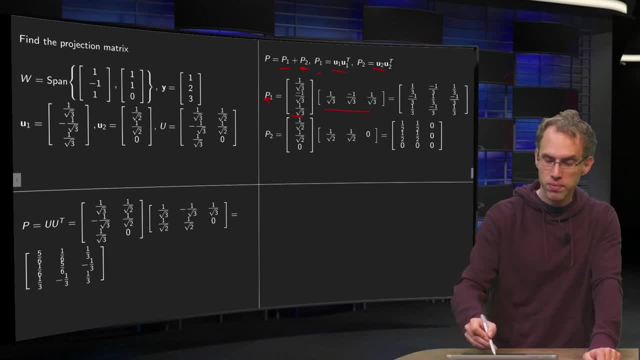 Again We can use row-column rule. So here we have our very short rows and very short columns. So now again, the first element, 1 over 3, second element, minus 1 over 3, third element: 1 over 3.. 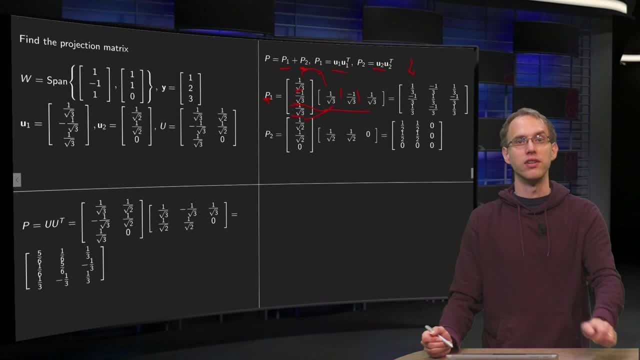 There you have the first column, and you can do the second and third column yourself. Similarly for p2, but now you use u2.. Here you have u2, u2, transpose, And again we use row-column rule. The product 1 over square root of 2 gives you the 1 half. 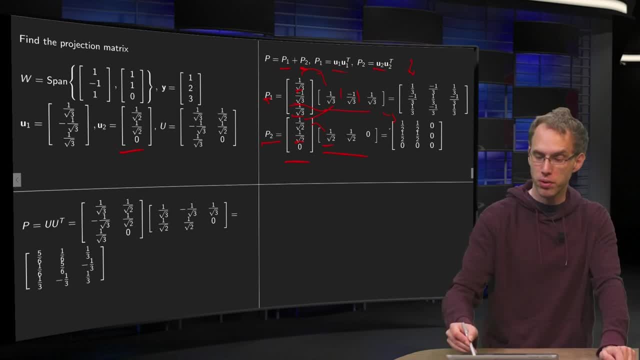 The product. 1 over square root of 2 times 1 over square root of 2 gives you another 1 half, And then 0 times 1 over square root of 2 gives you your 0.. Now you can do second and third column yourself. 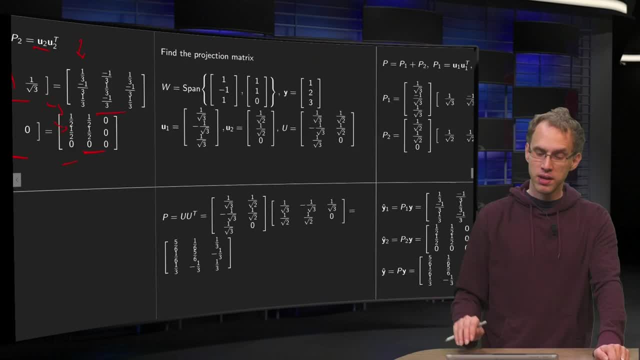 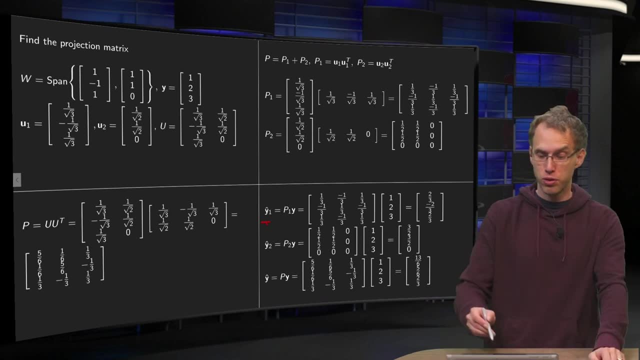 So there you have the p1 and the p2.. Now you can compute some projections. Let's compute the projection y hat 1, the projection of y onto u1.. We can do that now using your matrix p1.. So we have p1 and p2..